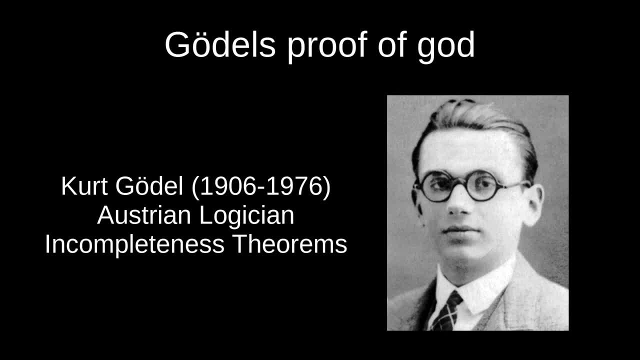 Hello world, My name is Viktor Engelmann. Welcome back to my channel. Today I want to do something that might seem off topic for my channel, but logic is an important mathematical foundation of computer science and I myself come from a background in formal logics. 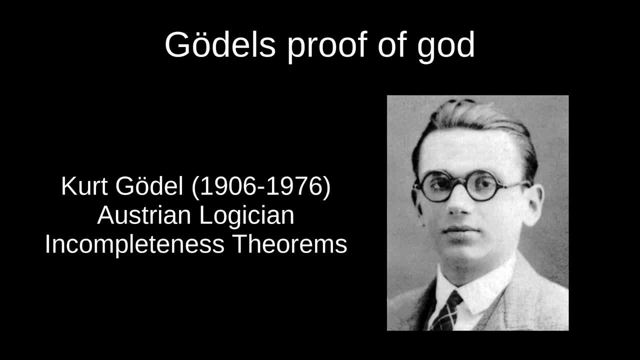 so it is not that off topic to talk about Gödel's god proof here. Kurt Gödel was an Austrian logician. He was one of the greatest, if not the greatest, logician of all time. His incompleteness theorems have been groundbreaking discoveries that have revolutionized. 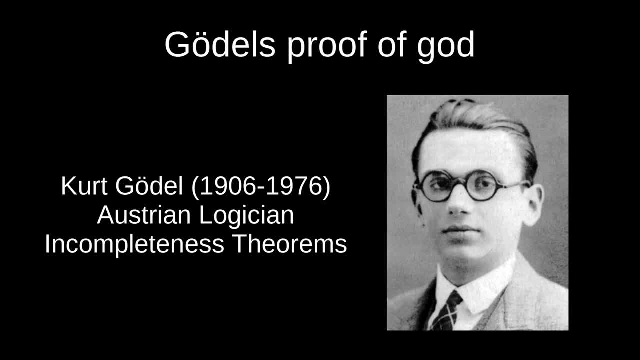 all of math, His proof of God. well, first of all, this is not really his proof. He took the ontological proof by Anselm of Canterbury and translated it into the language of modal logic, In case you don't know Canterbury's argument. his argument was that existence is something positive. 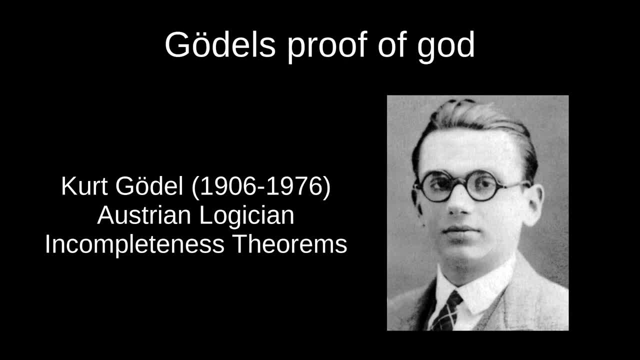 and if we define God as a being than which no greater can be conceived, then that must possess this existence property. His argument failed on every level because he had no understanding of logic and relational algebra at all. For one thing, his definition defines God as a maximal element, but then he uses this God as if. 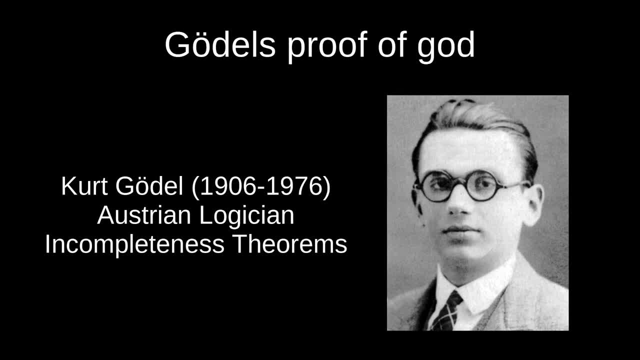 it was a maximum. In other words, God is a maximal element of a relation that he didn't define, that he didn't show to be acyclic or to even have a maximum or maximal element in the first place. Gödel at least fixed these issues. Gödel didn't publish the proof, though. 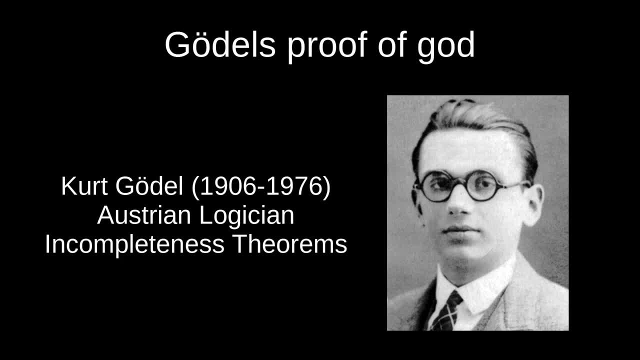 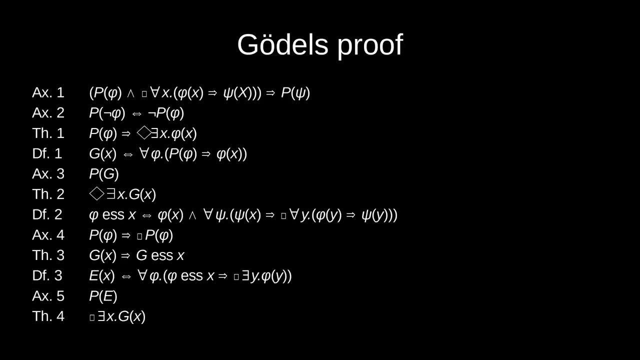 because he didn't want people to think he believed in God, Although, according to Hao, Wang, Gödel's wife has said that he did believe in God. When you look up the proof on Wikipedia, you see a quite intimidating collection of mathematical symbols that you most likely. 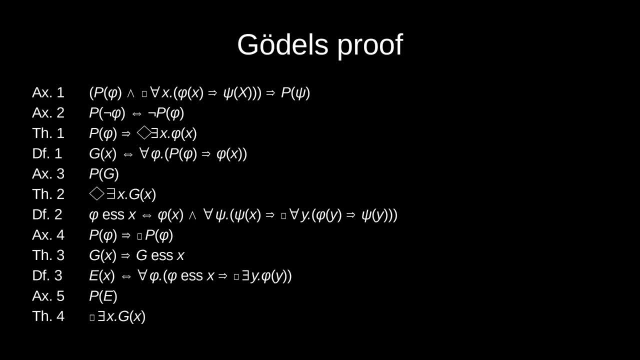 have never, ever seen in your life. Don't worry, we will go through this step by step, and if you have some understanding of math, I'm optimistic that you will understand the proof and every symbol here on screen will make at least some sense to you in the end. 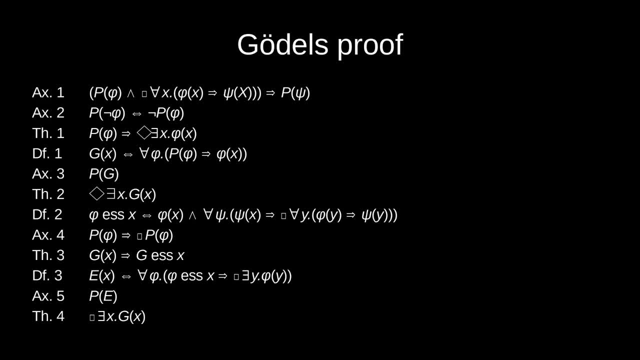 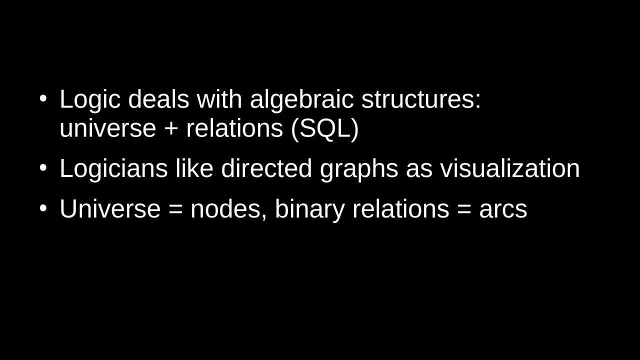 You may need to watch this video two or three times. I'd suggest to do that on separate days. Now, how do we approach this? This is a work of a logician. Logicians deal with algebraic structures, and this means that we have a class called a universe. 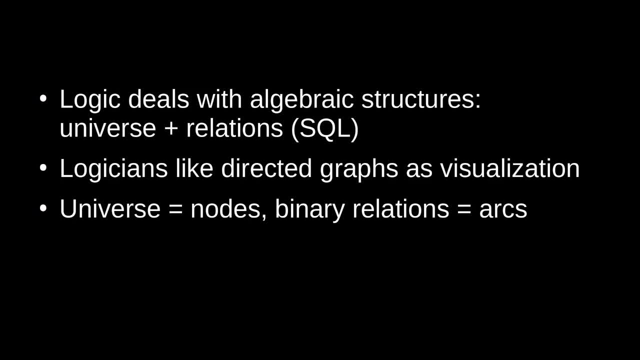 and the things in that universe have connections called relations. If you think of relational databases like SQL, now you are right. This is the mathematical foundation of relational databases. We logicians like to visualize algebraic structures using directed graphs, where we use little dots to represent the things in the universe. 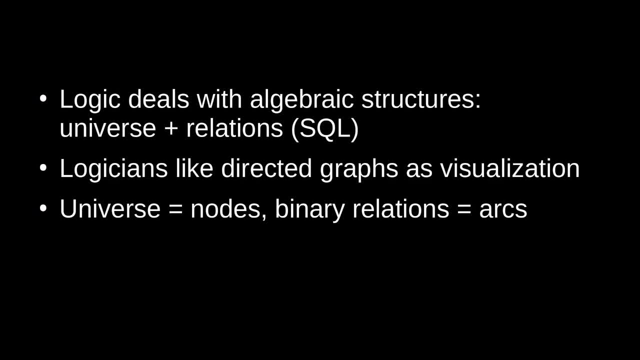 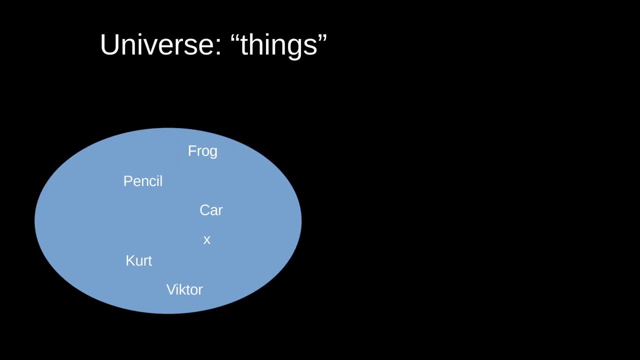 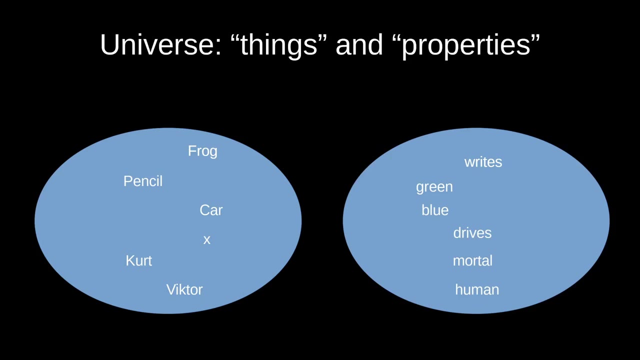 and arrows between them to represent the relations between them, if possible. So let's create such a universe with a few things in them: A frog, a pencil, me and Kurt Gödel, and a car In Gödel's model. we also think of properties as things in the universe. 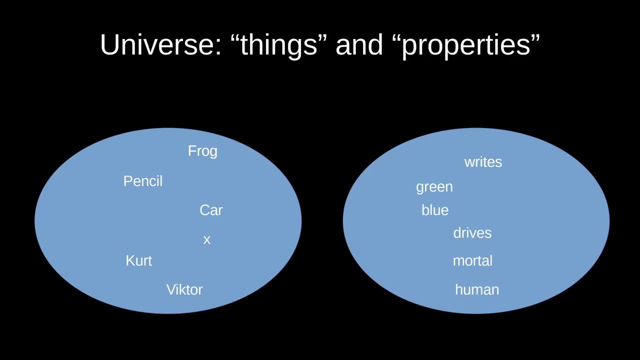 To illustrate that they have a different type. in a sense, I put them over here on the right And now I add arrows from things to the properties that these things have. Frogs are green, for example, My pencil is also green, and so on. 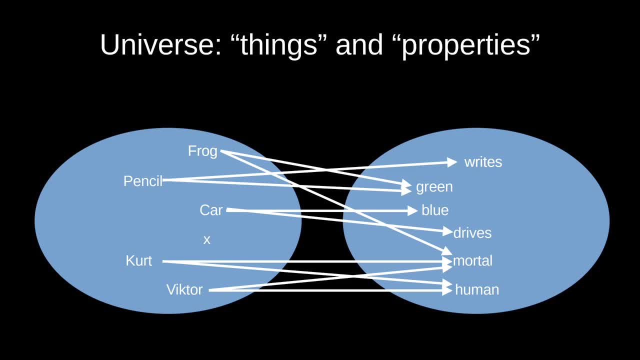 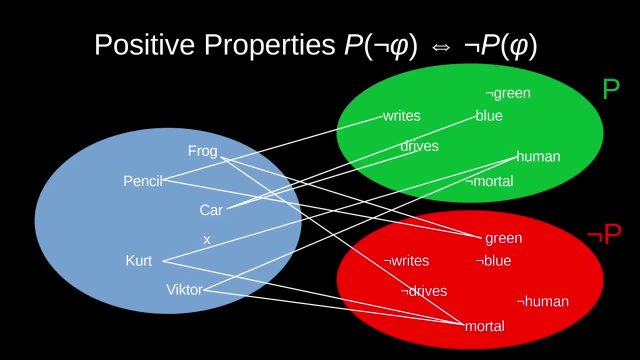 Okay, so far I think this is quite simple. Now Gödel divides the properties into positive and not positive properties. This might already remind you of Canterbury's argument. Axiom 2 now tells us that every property named phi- this here is the Greek letter phi- 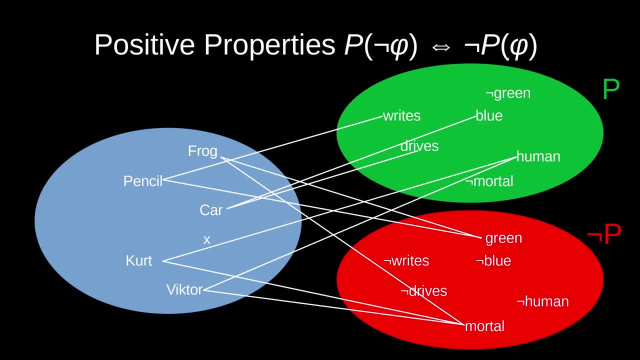 every property is either positive p of phi, or if it's not positive, then its opposite, not phi, must be positive. So these two sets down here of properties mirror each other. Okay, I like blue, so blue is positive. 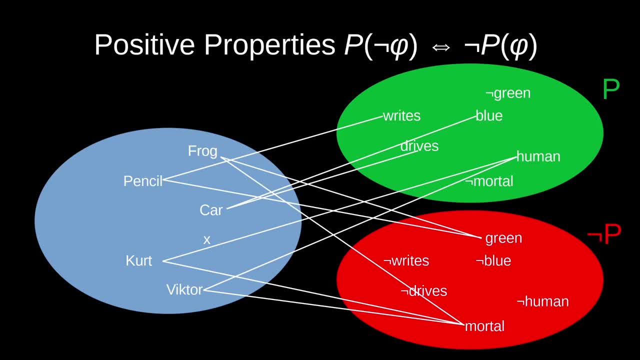 I don't like green, so green is not positive And not green is positive. in return, A car is only useful when it drives, so driving is positive. A pencil is only useful when it writes, so writing is positive. As a human myself, I'd say it's positive to be human. 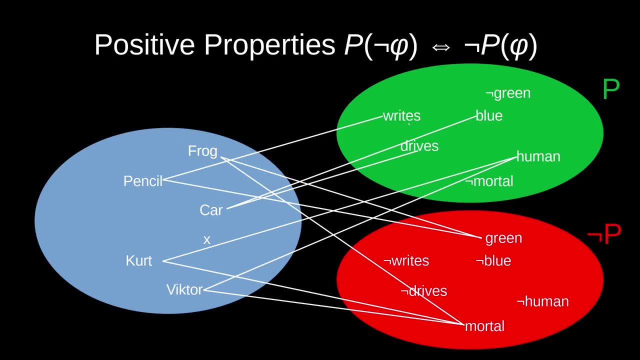 and most humans would prefer immortality. so I made mortality not positive down here. But wait, If you prefer green over blue. if someone stole my car, I'd rather it didn't drive. If humans weren't mortal, we'd soon be overpopulated. 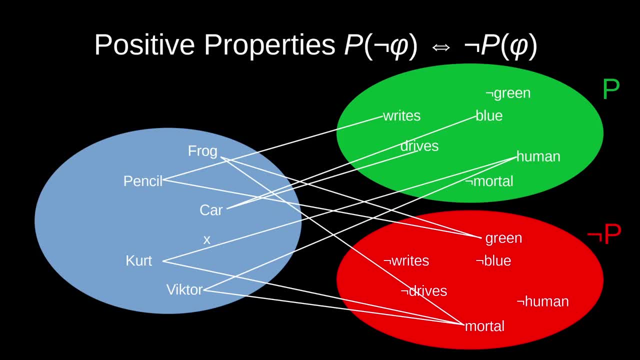 and be too loud, and God Enlil would send his storm, god Adad, to flood the entire earth, And that wouldn't work because, being immortal, we'd survive that even without Enki telling us to build an ark. So it is arguable what we should or shouldn't count as positive. 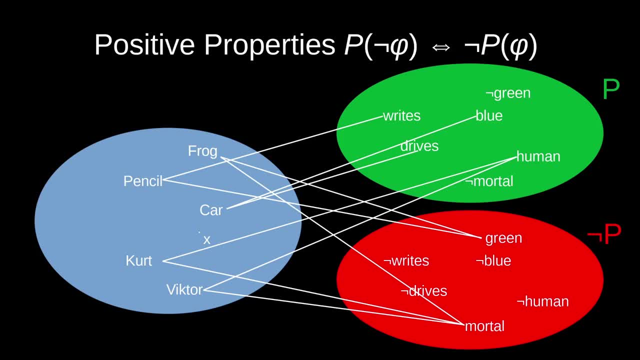 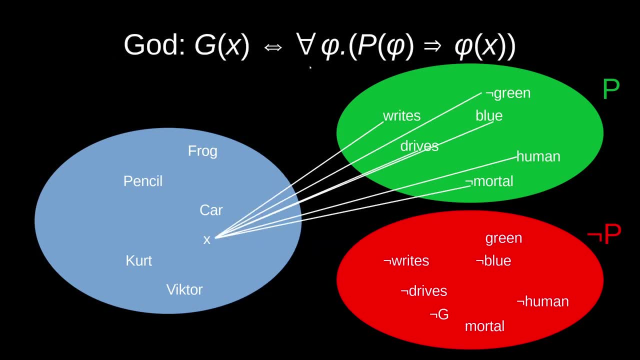 This x over here. this is what we will try to show to be God. Gödel defines a God as something that has all positive properties. That's definition. one A thing: x is godlike, g if and only if, all properties. 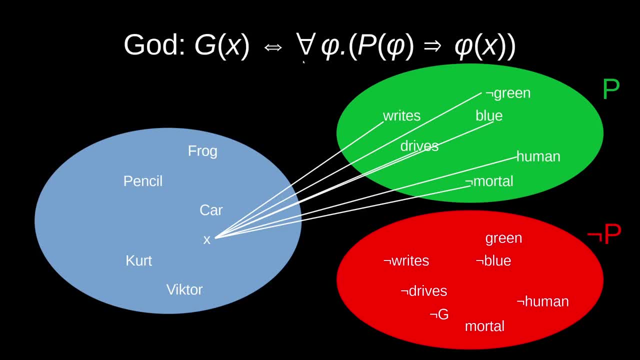 this upside down: a means all. so x is godlike if, and only if, all properties phi that are positive are also properties of this x. This here means x has this property when it is positive. So this is what this God would look like. 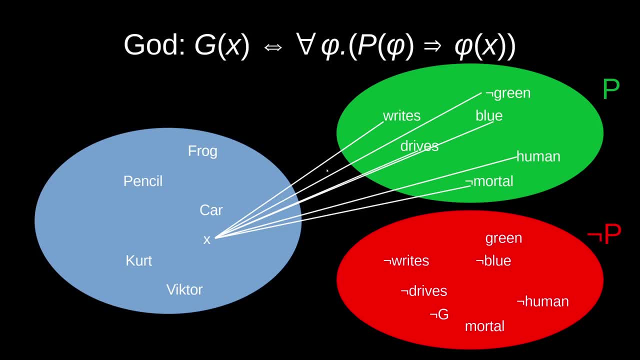 down here. Oops, I'm afraid I have just violated the second commandment And we have colored God blue. Okay, And God is human. Hooray, Christians, rejoice. We have proven Jesus by arbitrarily declaring humanity to be positive, This property of being godlike. 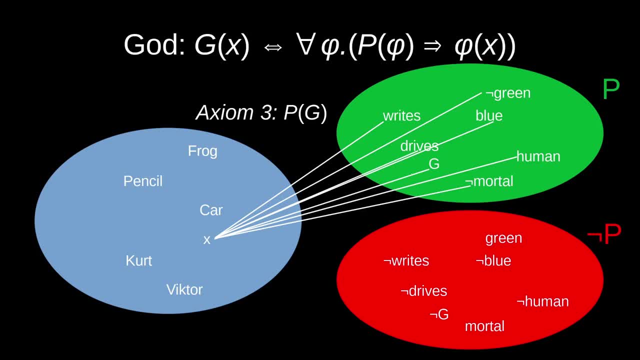 is denoted g, And axiom three simply defines this as a positive property. I don't know which God Gödel was thinking of, but given all the atrocities God Jahwe commits and commands in the Bible- genocide, human sacrifice, child murder, rape- 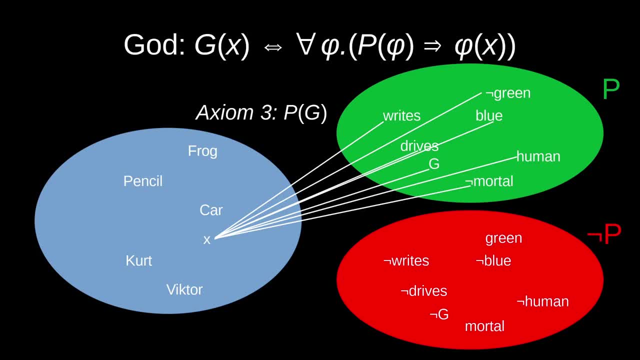 I'd be hesitant to call that a positive property. On the other hand, this definition, via having all positive properties, is a good justification for this definition. It just excludes evil monsters like Thanos or Jahwe. We don't know yet whether such an X exists in the first place. okay, 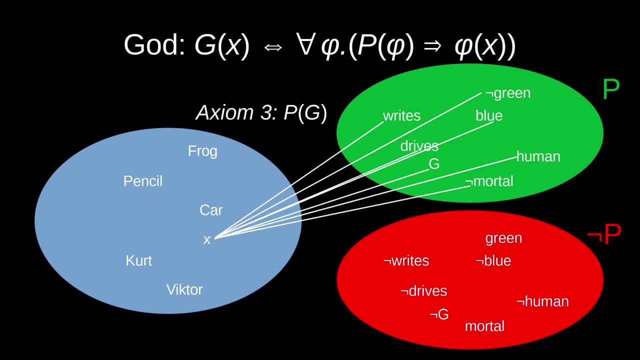 If something does have all these positive properties. this is what we will try to show. But what if God is partially blue and partially green? Then God would also have some negative properties down here. If we would allow this, then we could construct a counterexample to theorem three. 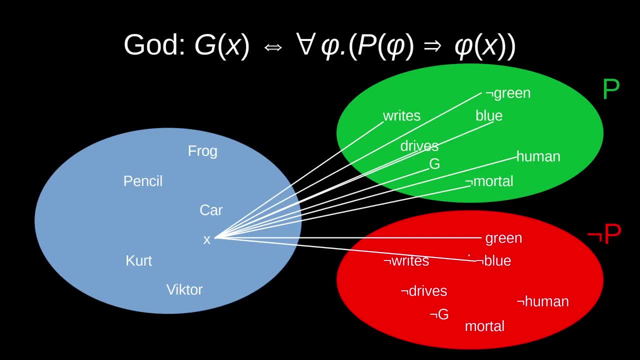 by having different gods with different negative properties. So this must be excluded. But Gödel did not exclude it. I'd say this is a mistake in its proof. but we can fix that with an additional axiom that says: if you have a property X. 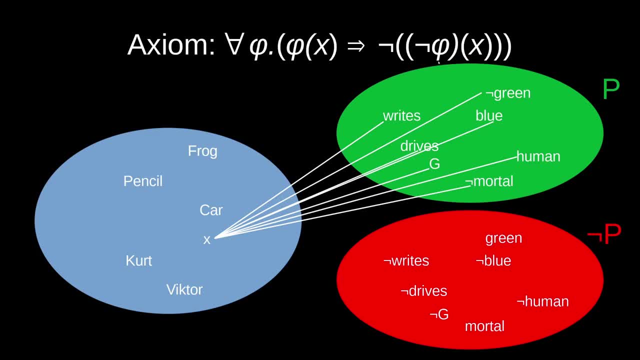 then you cannot have the opposite property. okay, Although I think Gödel assumes these properties to be modal logic formulas and then this follows automatically. Well, I am lazy, and some days I'm really eager, So I'd say in reality, 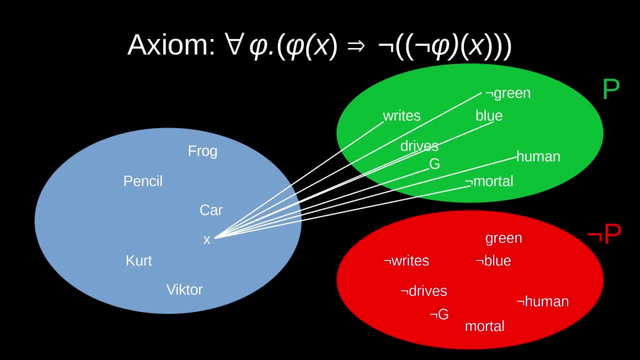 it's possible to have a property and its opposite. But, as I said, without this theorem, three falls apart, and I don't mean that only the proof falls apart and we might find a different proof. No, the proposition actually becomes false. We can construct a counterexample. 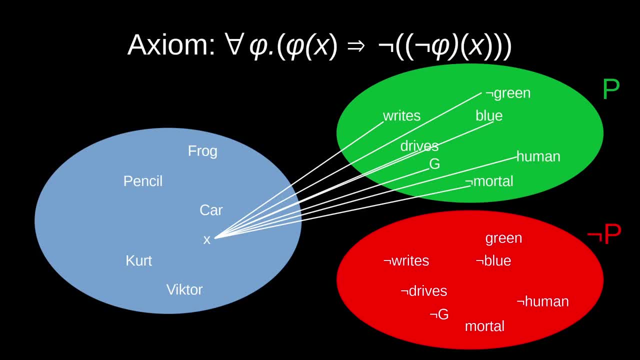 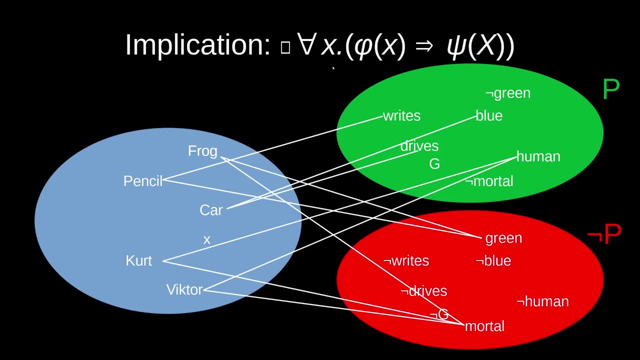 So we need to exclude this. Okay, moving on, Gödel doesn't define this separately, but he uses an implicit relation between properties. that I would call an implication. This box here is not a missing Unicode character in the font. This is a modal logic box operator. 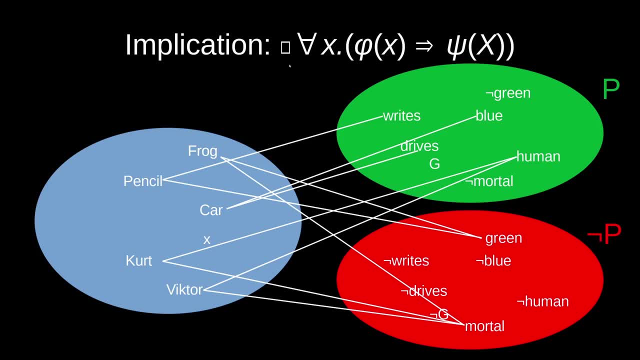 We will talk about this later. Just ignore it for now. What is an implication now? See, for example, humans. okay, We have two humans, Cord and Victor, and both of them are mortal. okay, So this we would call an implication. 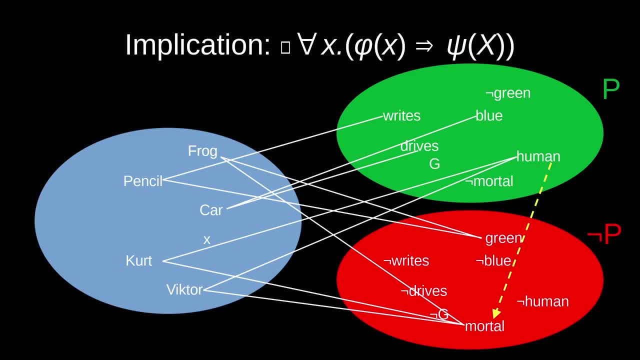 All humans are mortal, so mortality is a consequence of humanity. I represent this with this yellow arrow here. The other way around doesn't work, because frogs are also mortal, So we have a mortal thing that is not a human, okay. Therefore, mortality does not imply humanity, okay. 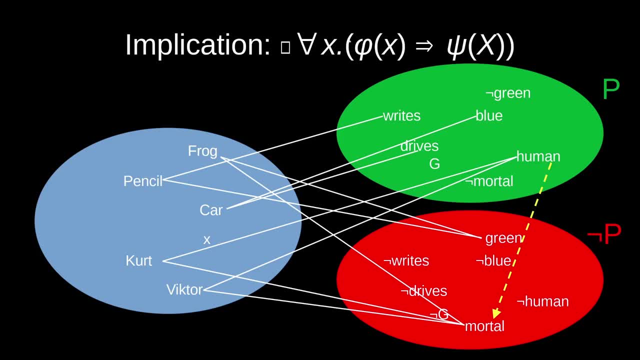 So property implies another property if all things that have the first property- human in this case- also have the second property- mortality in this case. In our little example universe, we get some funny effects. The only thing that writes is the pencil. 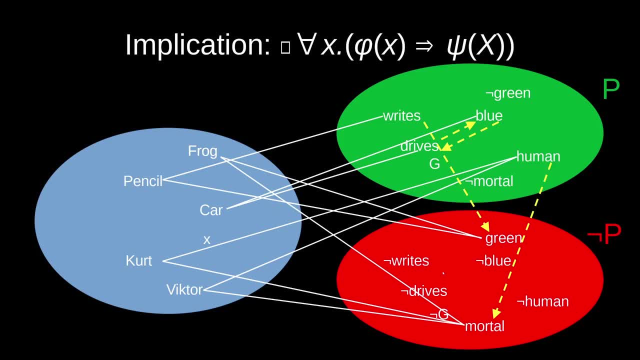 which is also green. So writing implies being green here, and the car makes driving, and blueness imply each other. Okay, let's live with that. Now, axiom one says that positive properties cannot imply negative properties. So if a property is positive, 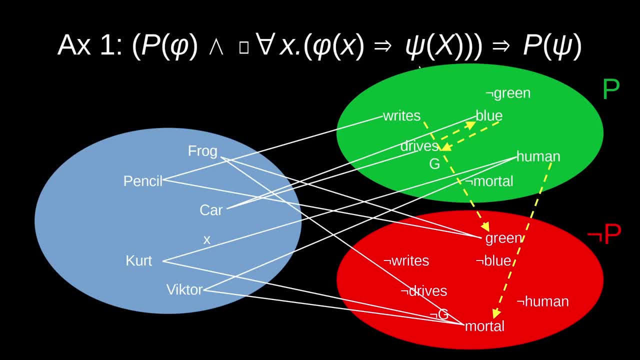 and this property phi implies a property psi. this here was the definition of the implication. then psi must also be positive. So these arrows- rights to green and human to mortal- are illegal. Yellow arrows within the green zone are okay within the red zone and even from red to green. 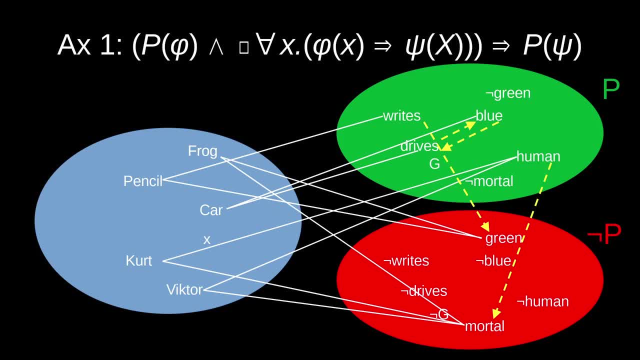 but not from green to red. okay, Maybe our assignment of properties to things is incorrect or our classification which properties are positive was incorrect. I mean, Adam and Eve ate an apple. Of course humanity is negative. Let me fix that There. 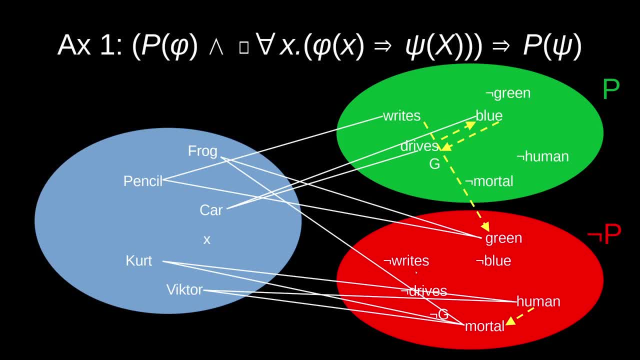 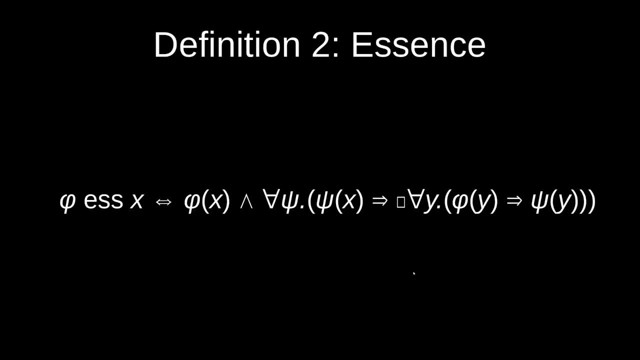 Okay, but now God absolutely can't be human anymore and we have disproven Jesus, Damn. Okay, let's talk about definition two, the essence. This is a very important but pretty complicated definition. Don't worry, we will decipher it step by step. 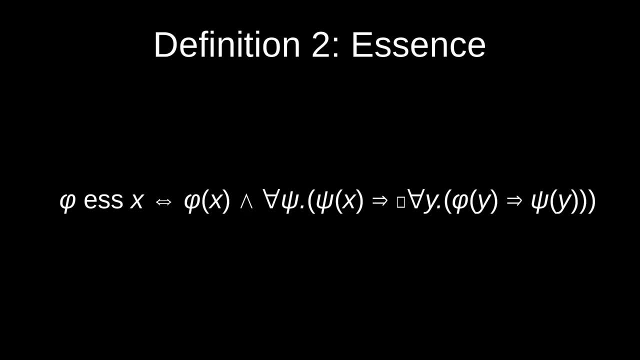 You might want to think of the essence as something that is the defining characteristic of something. The defining characteristic of a pencil is that you can write with it. for example, The defining characteristic of a car is that you can drive with it. The color of the pencil or the car. 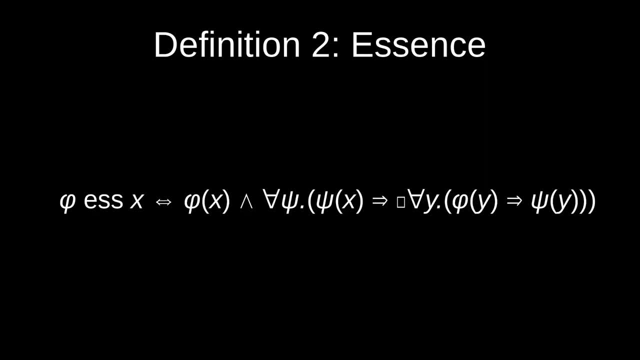 are secondary to that. Okay, so how does Gödel express this in the language of modal logic? A property phi is the essence of a thing, x, if and only if. Well, first of all, x must have that property phi, The defining characteristic of a car. 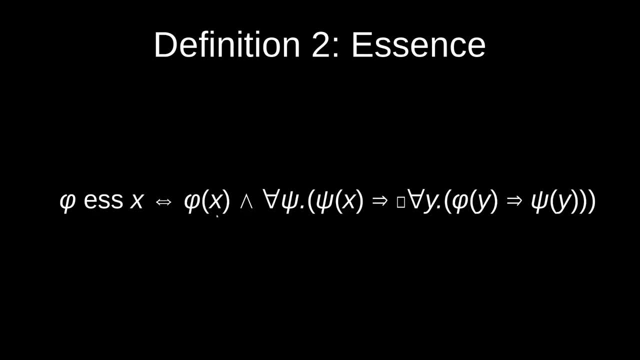 isn't that, you can write with it. So it must have that property and all other properties that it has must be implied. This was our definition. This was our definition of implication. So all the other properties phi must be implied by that essence. 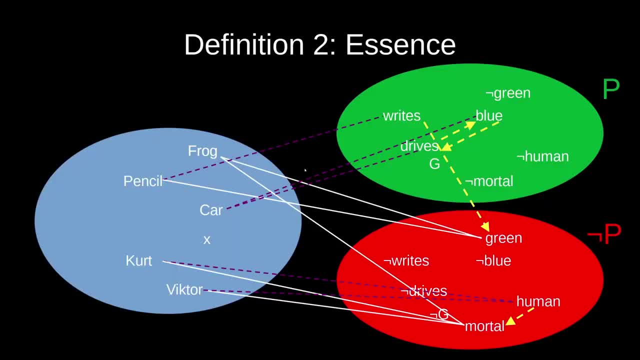 In our visual representation. we see, for example, that writing is the essence of the pencil, because its only other property, green, is implied by that Right. Pencil writes, The only other property green is implied, So writes is the essence. 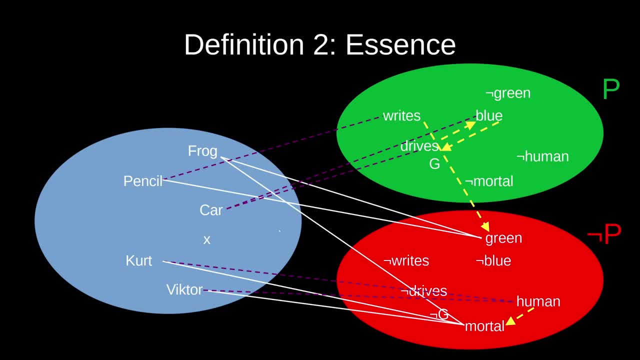 The essence of me and Kurt is humanity, because our only other property, mortality, is implied by that. The car has two essences: blue and drives, because these properties imply each other And the frog has no essence. That's also possible. 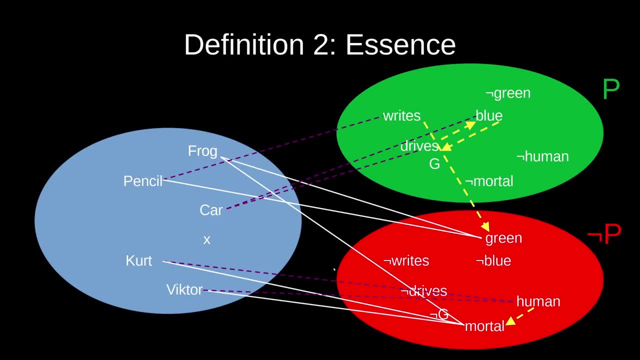 Green doesn't imply mortality and mortality doesn't imply green. But notice, if you have multiple essences they must imply each other, Like here, So they are in a way equivalent. Effectively you can have only one real essence. 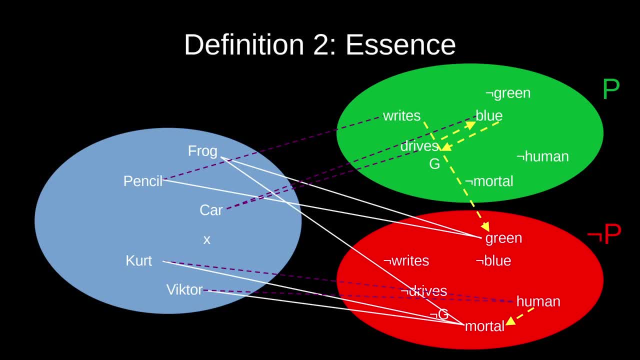 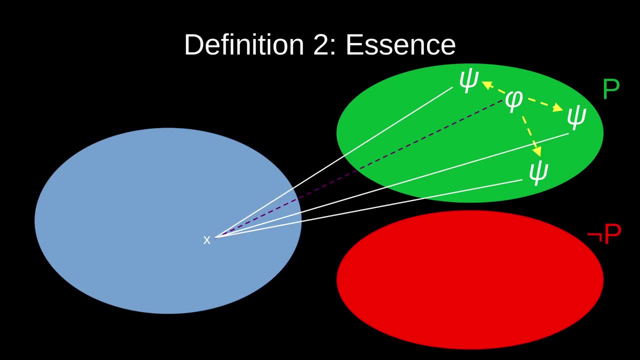 All other essences are redundant. So this is generally what essences look like. They are these central properties that imply all the other properties. The other properties can imply each other also, that's no problem. They can even also imply all the other properties. 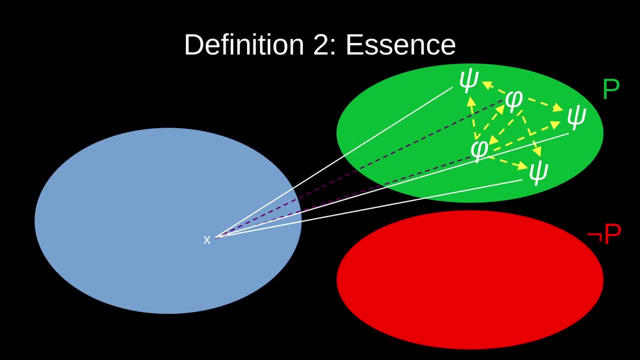 Then they are also essences, Like in the case of the car. Notice, when you have just one negative or neutral property down here, then your essence cannot be positive anymore, Because then the positive essence would have to imply the neutral property. That would be a yellow arrow from green to red. 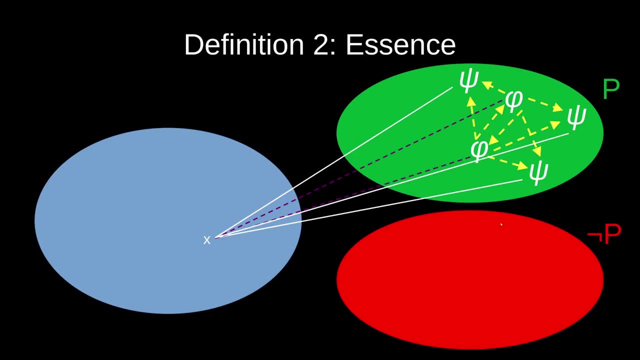 and that would violate axioms. You can have a negative essence but also have some positive properties. That's okay. I find that a terrible message. You are either 100% good or you are essentially bad, Rotten to the core. But argumentum ad consequentium. 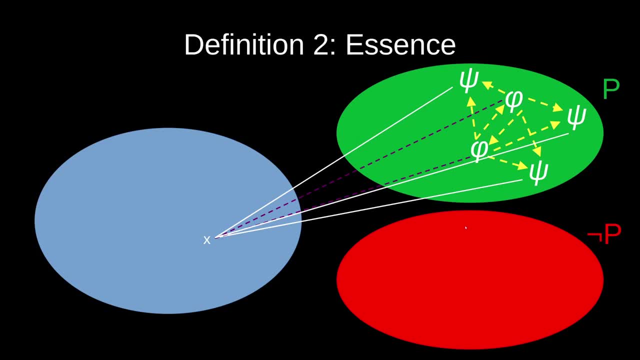 is not a valid argument, so we will accept that and move on. This definition of essence doesn't make much sense, frankly, because what if you have a green and a yellow pencil? Then neither green nor yellow are implied by the pencil's writing property. 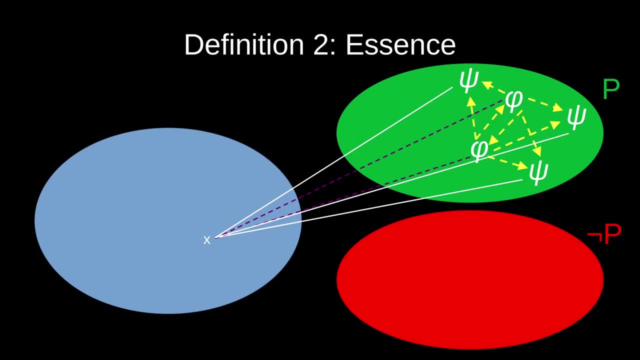 and then being able to write is not the essence of the pencil anymore. The pencils don't have essences anymore. I don't think an essence should be influenced by a minor property like the color of a pencil. But okay, Let's move on. 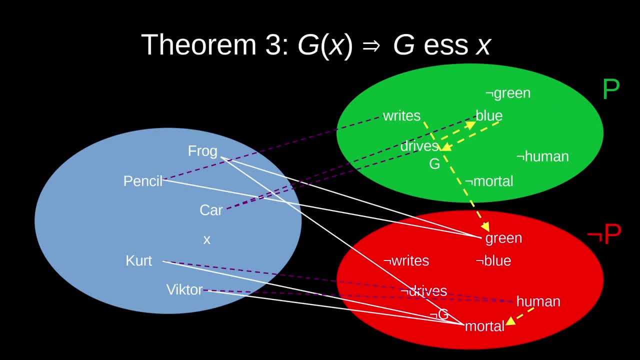 We haven't talked about Theorem 1 and 2 yet, but let's talk about Theorem 3 anyways. Theorem 3 says that if there is a god, X- X is a god now- then this godliness G is an essence of X. 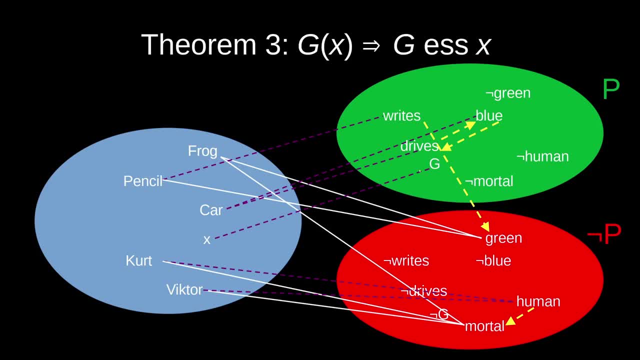 So this white line has become purple now, and that's what Theorem 3 says. The proof for this is rather trivial, Because how do we determine that G is the essence of X? All other properties of X must be implied by G. X has all positive properties. 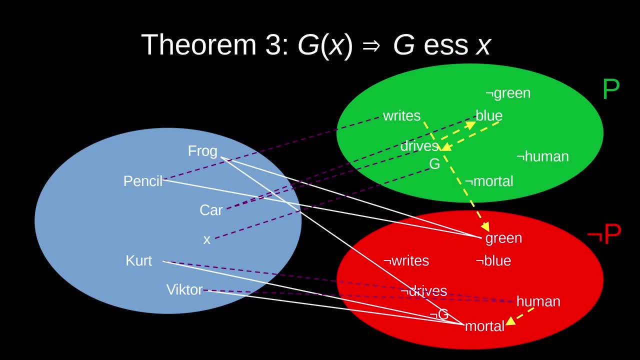 so we need to show that G implies all positive properties by definition, 2.. There, this is what we need to show. How do we show that? Well, how do we show that G implies immortality, for example, This yellow arrow down here. 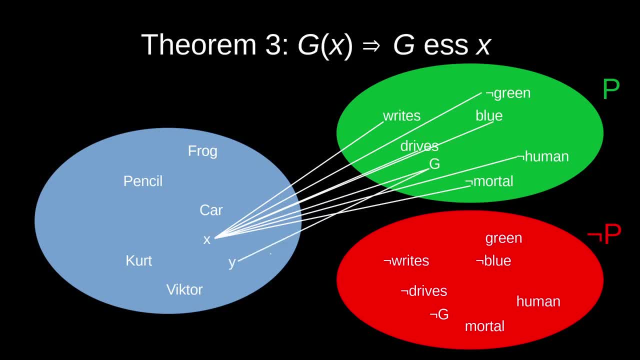 We need to show that all things that have property G, right Y, also has property G. now, all things that have property G must also be immortal. That's how implication was defined. So let's say X and Y are godlike. Then definition 1 again gives us that 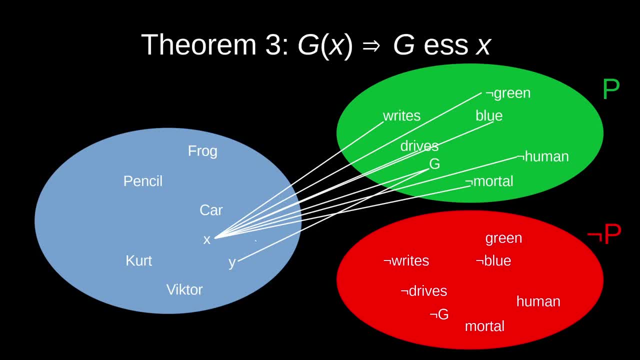 X and Y have all positive properties, including immortality, So Y is also immortal, And this works for all things that have G. So, yes, every godlike thing is immortal And G thus implies immortality, And the same argument works for all positive properties. 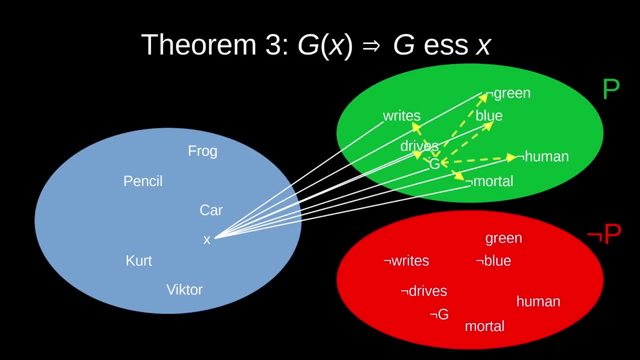 So G implies them also, And that's it. G implies all positive properties. We have yellow arrows from G to all positive properties, And that is the definition of G being the essence of X. That is what we had to show. This is what would fail. 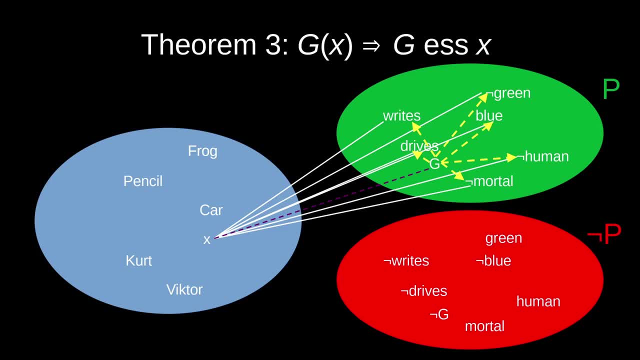 if we allowed X to have negative properties, Then that property would not be implied by G, because a yellow arrow from green to red would violate axiom 1. And that would violate the definition of G being an essence of X. Okay, this was quite heavy already. 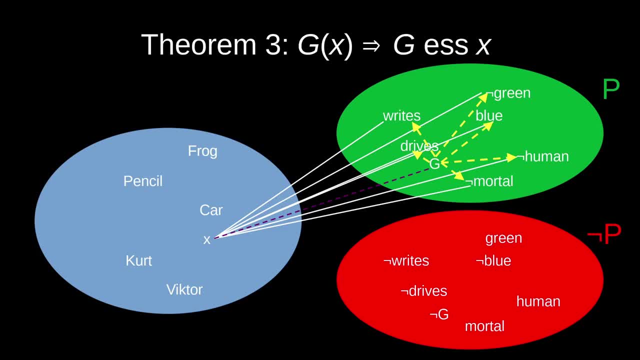 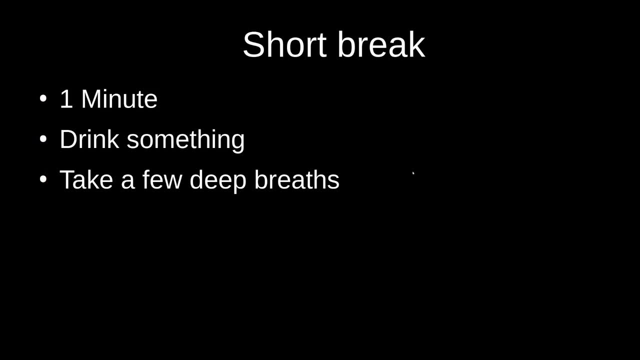 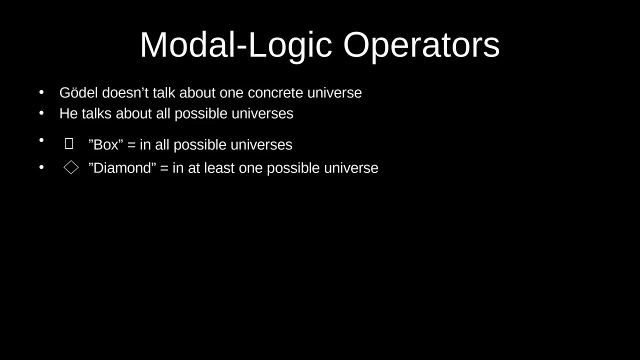 but we haven't even really started, So let's have a little break to take a breath. Alright, let's continue In the definition of the implication. we had seen this box symbol right. 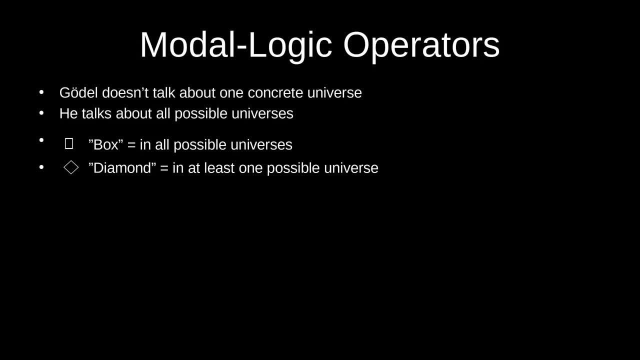 And I had told you to ignore that. but now we come back to that. So far I have simplified the things Gödel talks about. So far we had one concrete universe with things that, But Gödel actually talks about all possible universes. 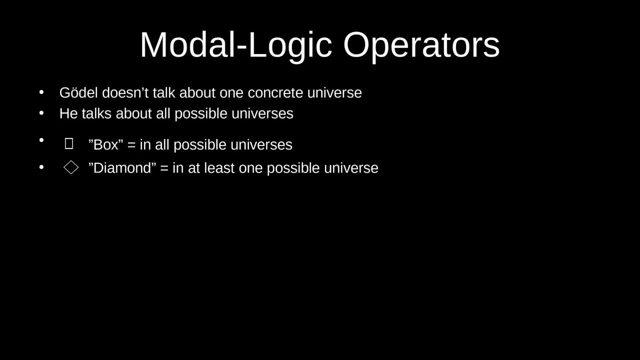 And that is what these box and diamond operators are for. Diamond phi means that the statement phi is true in at least one possible universe, And box phi means that the statement phi is true in all possible universes. Let's look at an example. 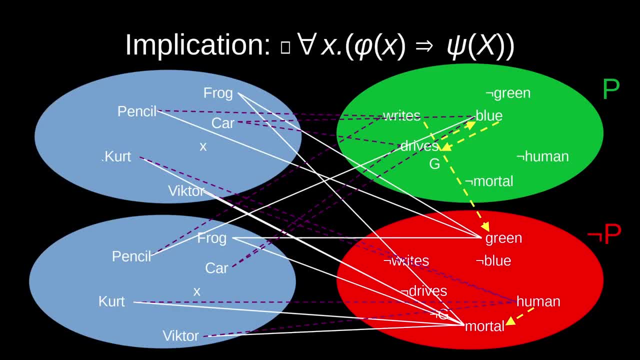 Instead of our one universe, we now have an infinite number of possible universes, but I don't have that much screen space, so only two universes have fit in here. The second universe is wildly different from the first one. In this bizarro universe, 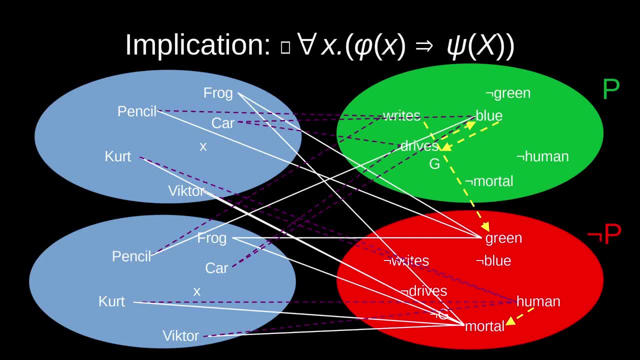 I have picked a blue pencil when I bought it last week And I bet Mr Spock has a beard off screen. Okay now what does this mean for implications? Implications now only remain if they hold true in all universes. For example, I now have a universe in which there is something that is blue. 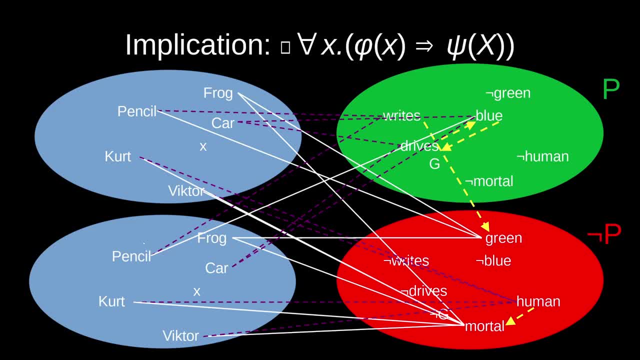 The pencil Right, But this thing doesn't drive. Therefore, blue isn't an essence of the car anymore. Also, I now have something that writes, but that isn't green, So green isn't implied by writing anymore. But that also means that writing isn't the essence of the pencil anymore. 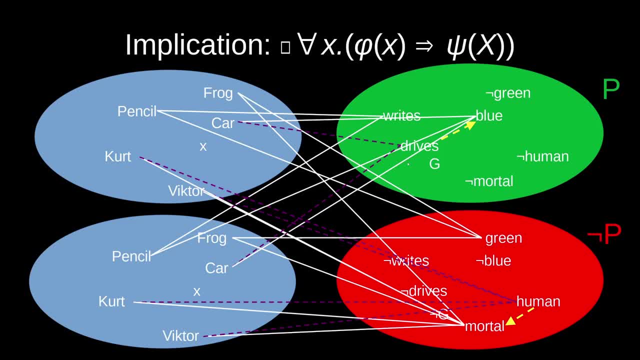 because the green pencil now has the property green, which isn't implied by writing anymore, And the same for the blue pencil. Seriously, Changing the color of a pencil from green to blue has changed the essence of blue cars? I don't think that should be possible with a good definition of essence. 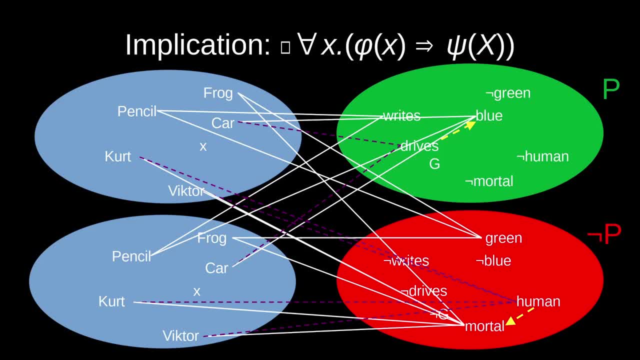 For as much as I admire Goethe, this is a really, really bad definition, Because everything, or at least almost everything, can have different properties in different universes. So then nothing satisfies this implication across all universes, So nothing implies anything anymore. 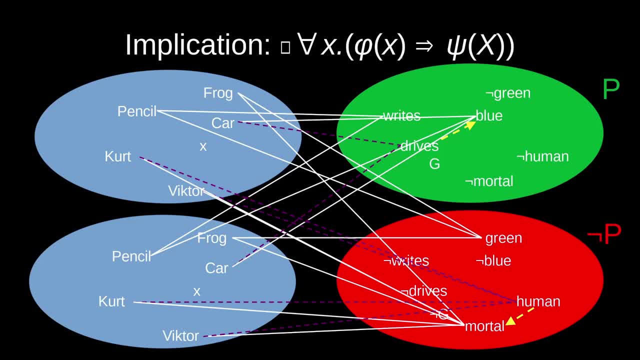 And then everything has properties that aren't implied by each other, And then nothing has an essence. I think the whole model collapses into a meaningless set of lines at this point. In my opinion, an essence should be an indispensable property, a property that you have in each universe in which you exist. 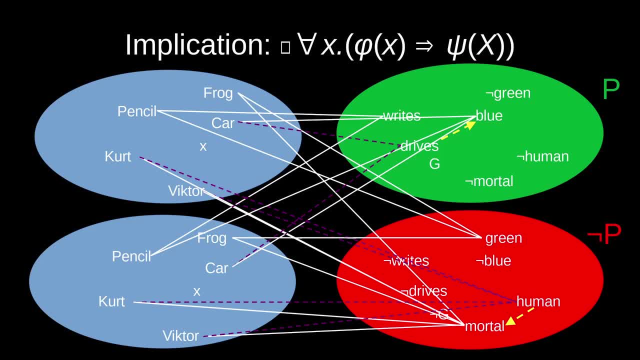 But that would be a completely different can of worms. The only reason for Goethe's definition seems to be that this definition makes godliness an essence of gods, which he later needs. But okay, let's move on. But I do remark that Goethe is using contrived definitions. 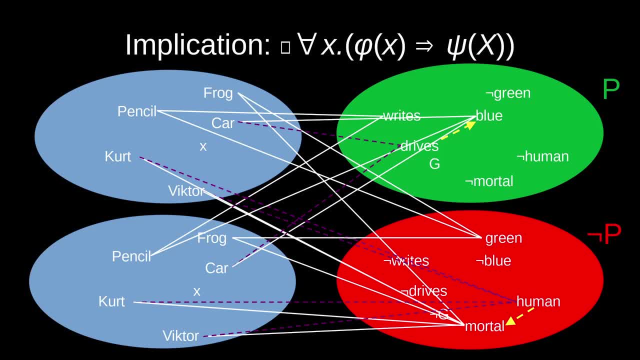 to force a desired conclusion. Now let's talk about theorem 1. It says that for every positive property, phi, there must be at least one universe in which a thing exists that has this property. So every property in the green zone must have a neighbor in some universe. 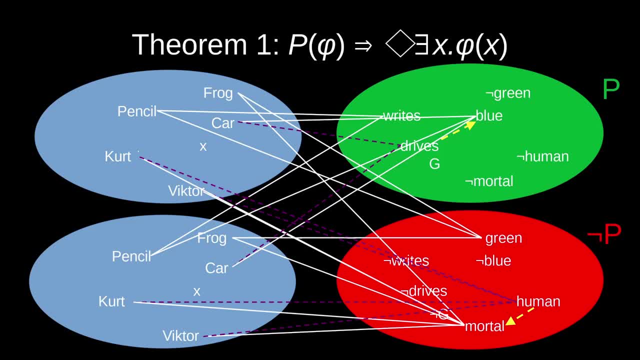 Goethe calls this a theorem. A theorem would be a conclusion from the axioms, But mathematically there is no reason at all to just throw some lonely property in there. You could argue that if nothing has this property, then this property is useless. 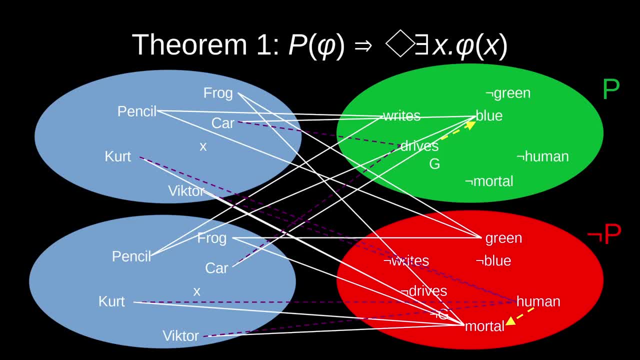 and useless properties cannot be positive, only neutral. But that's a philosophical argument. That's your interpretation of what p stands for, not what p's formal definition logically entails. So I'm sorry, but I'm downgrading theorem 1 to an axiom t1.. 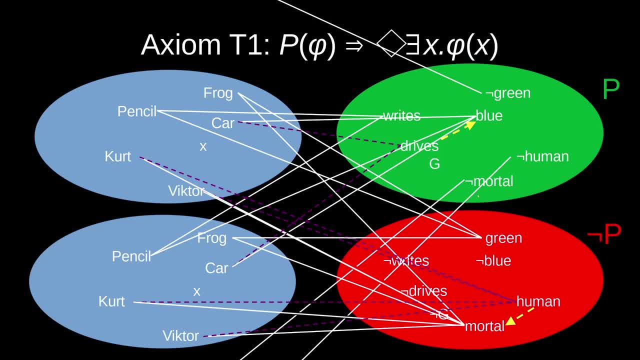 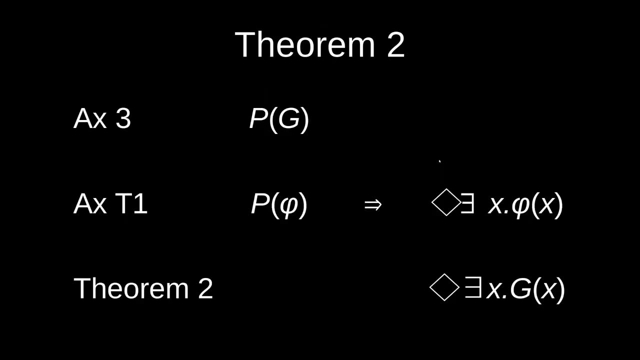 And yeah, now everything in the green zone has some neighbor somewhere. And why is that important? Why do we have that? Well, remember that we had defined g to be positive, And that is precisely what we use this theorem for. Axiom 3 says g is positive. 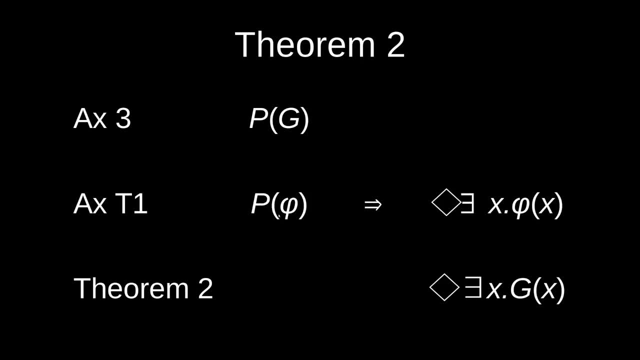 So we can apply axiom t1 to it, replacing phi with g, and conclude that there possibly exists something that is a god Great. We have proven that in some possible universe a god exists, or, using Goethe's language, it is possible that god exists in our universe. 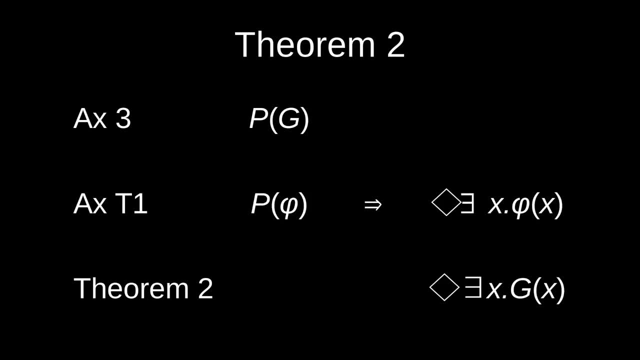 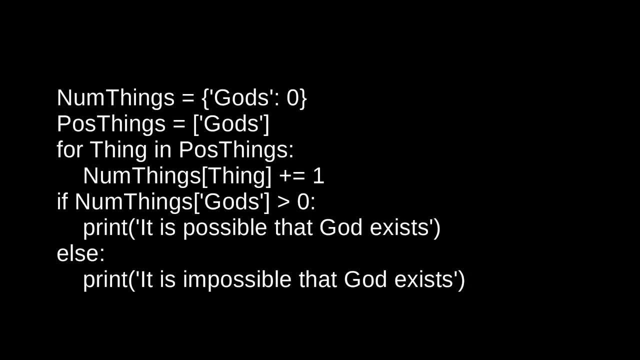 And we only needed two completely contrived axioms that were obviously designed to produce this exact outcome. I might as well say that this Python program proves the possibility of god. This is exactly what we have done here, just written in Python, instead of modal logic. 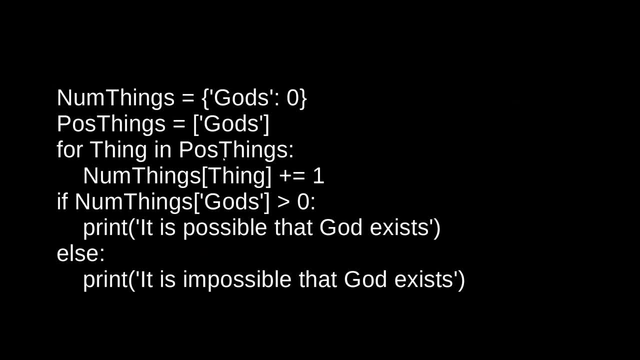 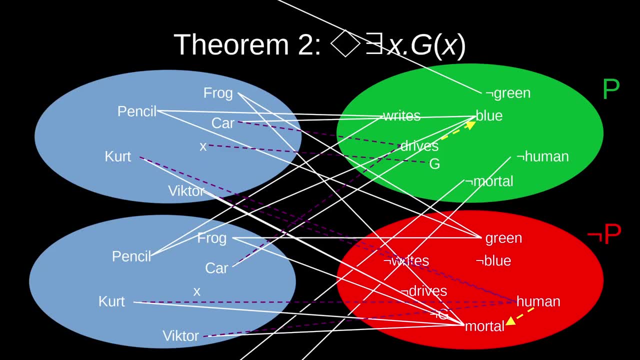 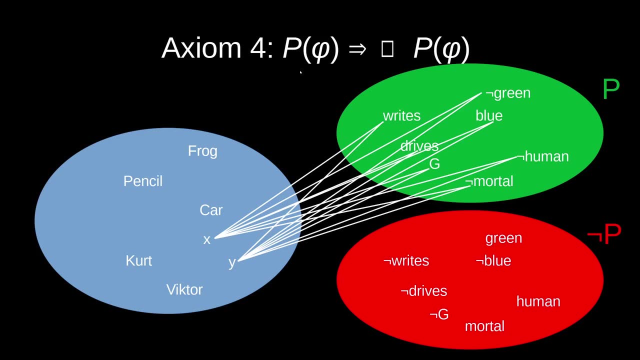 But what this gives us now is the information that in some universe there is a god x and godliness is its essence. Okay, now let's look at axiom 4. Positive properties, phi, are necessarily positive. If it makes you happy, you have my permission to interpret this. 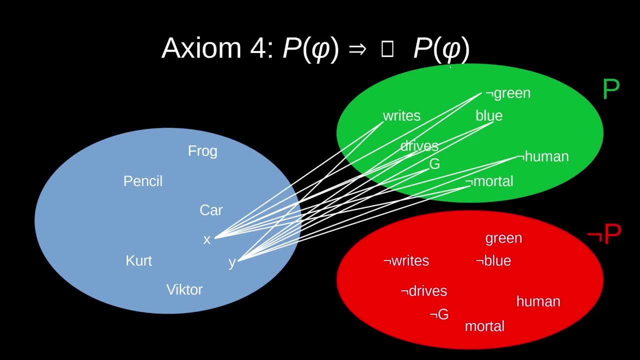 as p being an objective morality. Mind you, we don't prove that morality is objective. We assume it to be objective because otherwise the proof falls apart again. We need this assumption to make theorem 3 work with multiple universes. Think back to theorem 3.. 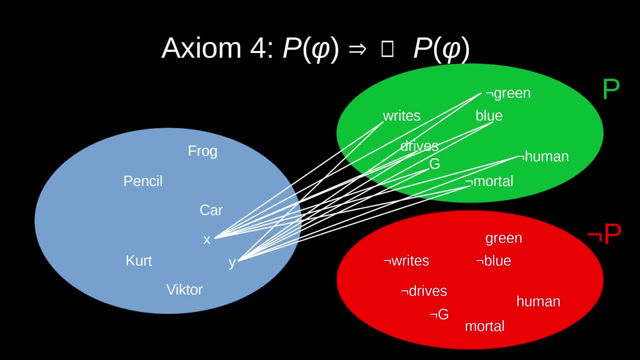 We used the fact that all gods have all positive properties, and that wouldn't even make sense if this positivity wasn't something objective. So we use that gods have all positive properties to prove that all positive properties follow from godliness, which then meant that godliness is an essence of god. 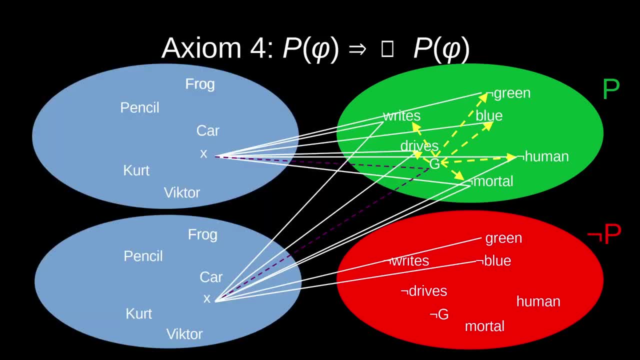 If we allowed different universes to have different interpretations of what properties are positive, then, yeah, gods from different universes would have, or could have, different properties. Say the universe down here green is preferred over blue, Then the implications aren't consistent across universes. 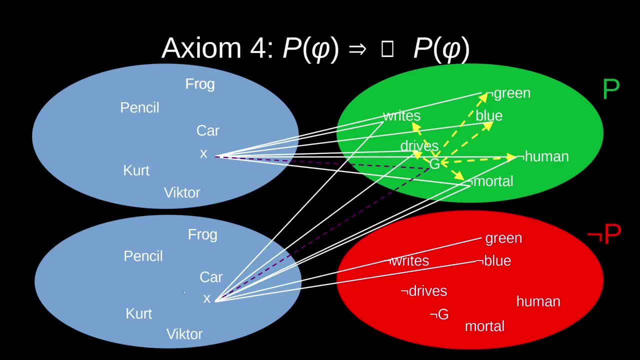 The x down here is a god, but not blue, right? So blue doesn't follow from godliness anymore. And then this god up here has a property- blue- that is not implied by godliness, And then godliness is not an essence of this god up here anymore. 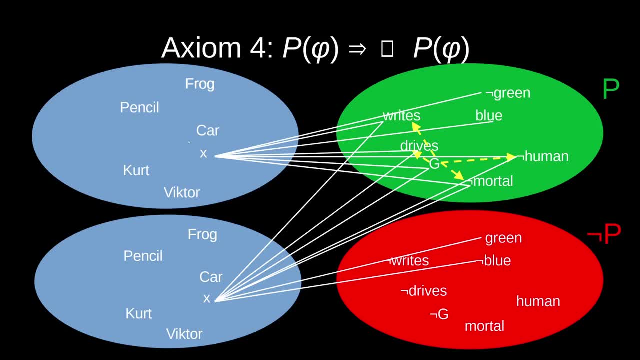 And then the proof doesn't work anymore, because in theorem 4 we use that g is an essence of gods. Phew, this was a lot. Let's take another one-minute break. Drink something, have a deep breath. We are almost through. 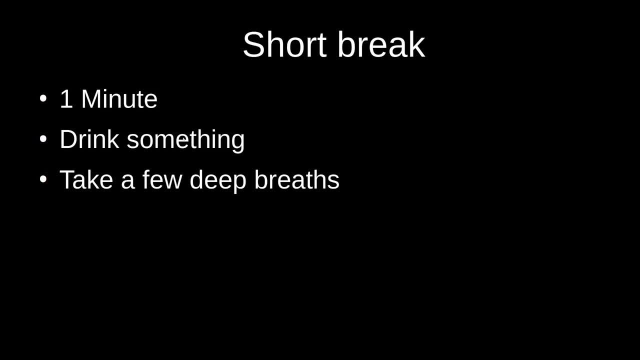 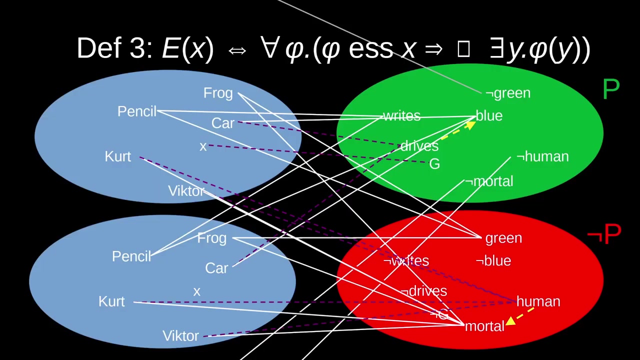 Again. if you don't understand everything, you can watch this video a second time, a third time Again. I'd suggest to do that on separate days. Thank you for watching. See you next time. Bye, Okay, now let's come to the final three lines of the proof. 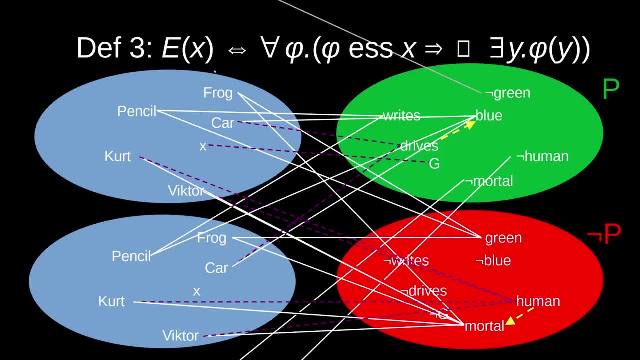 Definition 3 defines so-called necessary existence, defined with the letter e over. here The definition is a bit intimidating again, but don't worry, it's not that terrible, I promise. This says that a thing x necessarily exists if all of its essences, all essences of it. 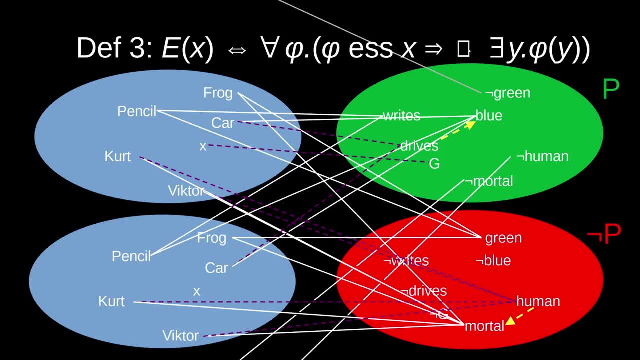 are realized in all universes. Box means all universes. In each universe there exists something that has this property. Let me repeat that a bit slower: A thing, x like this god we have found here, necessarily exists if and only if. all properties. 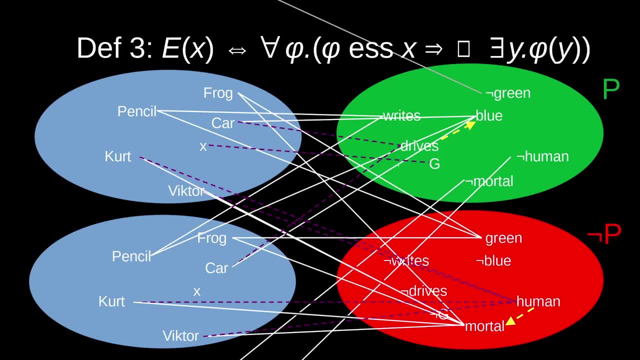 that are essences of x. so in our case, this g exists in all universes. Box was: all universes. In all universes there exists something that has this property g, And this is what we want to prove in the end, right? 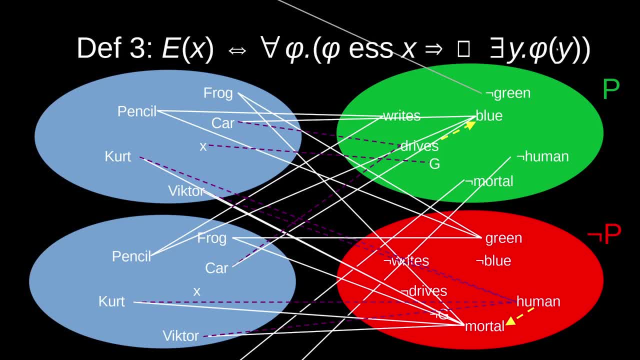 That in each possible universe there is a god, But oh my x having property g. how should we prove such a complicated thing in the few minutes that are left in this video? We don't. Why should we prove anything? We just define this into existence, again with axiom 5.. 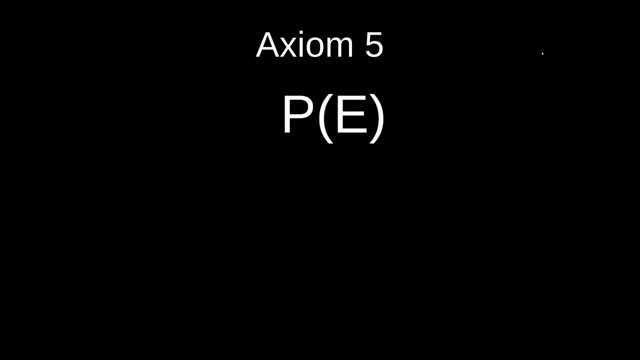 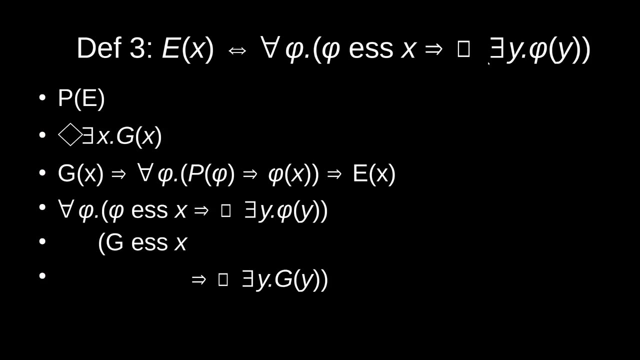 Necessary existence is positive. Yippee-ki-yay, And then we get everything for free again. Necessary existence is positive. Remember Ansem of Canterbury. Necessary existence is positive. We already have found a god x in some universe. Because that thing is a god, it has all positive properties. 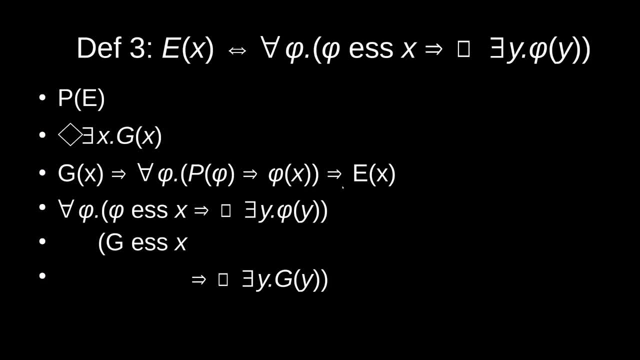 And yeah, since e is now positive, this includes necessary existence. And yeah, this complicated stuff that you worried about is not what we need to prove. No, this is what we now get for free. We get that all of x's essences. 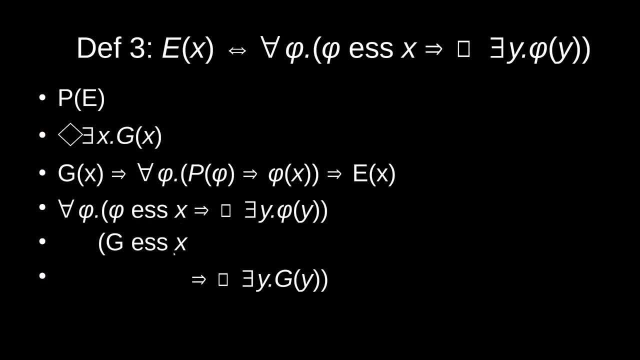 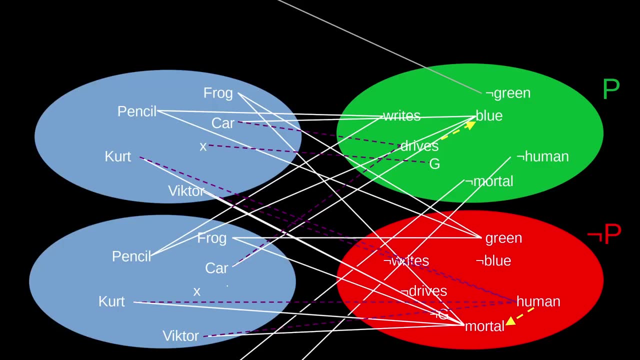 in particular, g being an essence of x. g now exists in each possible universe. In each possible universe there exists something that is a god. So in our very convoluted diagram we now get that all possible universes have a god. You see down here. this now also has a god. 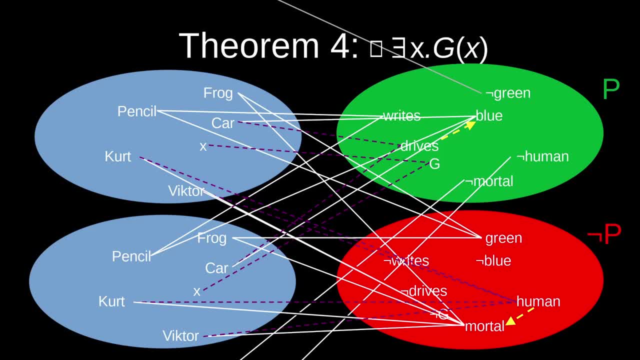 And all the other off-screen universes also, And this is exactly theorem 4.. Necessarily, there exists something that is a god. This is all. That is Gödel's proof of god. Okay, let me recap Gödel's proof. 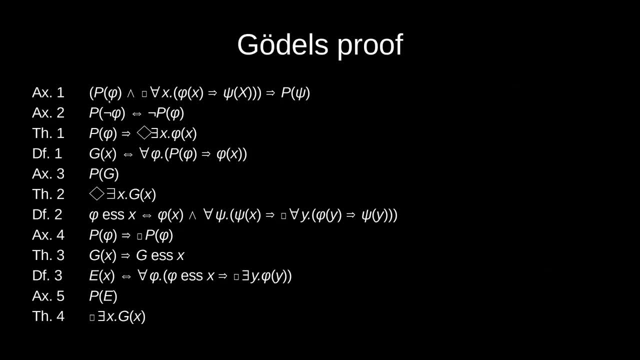 Axiom 1 said that positive properties imply only positive properties, So the yellow arrows cannot go from green to red. Axiom 2 said that properties are either positive or the opposite is positive, which meant that the red and the green zone mirror each other. 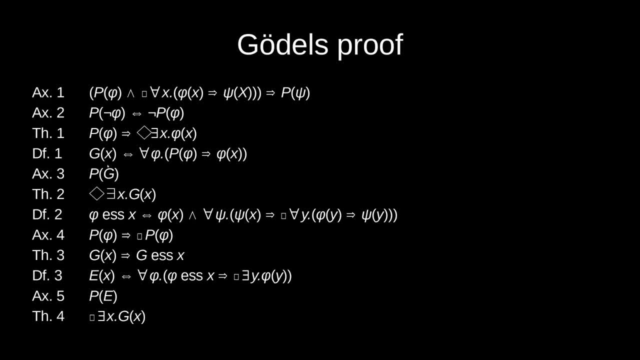 Definition 1 said that something is godlike if, and only if, it has all positive properties. Theorem 1- that I downgraded to an axiom T1, said that positive properties must be realized somewhere. So in some possible universe there needs to be an x that has that property. 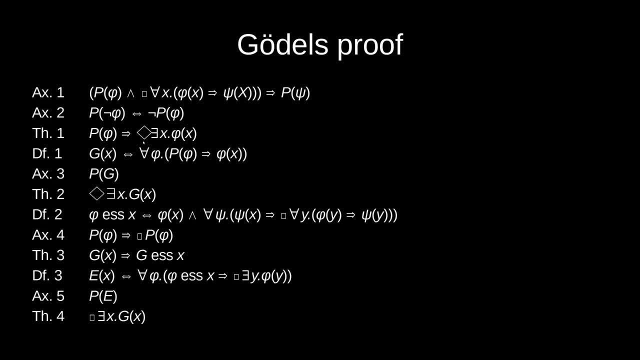 And why did we have that? Well, for the very simple reason that, using axiom 3, defining godliness as positive, we can put this p of g into this p of phi, replacing phi with g, And then we get: Possibly exists a god, and that's theorem 2.. 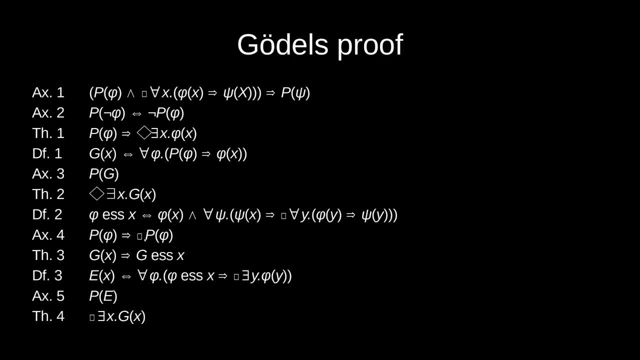 Definition 2 defined an essence of something as a property that implies all other properties of that thing, These purple dotted lines, Axiom 4, enforced the definition of positive properties across all universes, what we called objective morality. That was a technical detail we needed for theorem 3 to work across multiple universes. 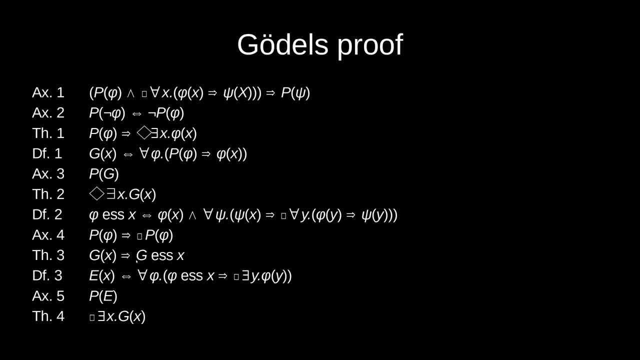 Theorem 3 said that godliness, g is an essence of gods. All gods, everything that has g has all positive properties. Therefore, g implies all positive properties. So g implies all properties of gods and is thus an essence of gods. 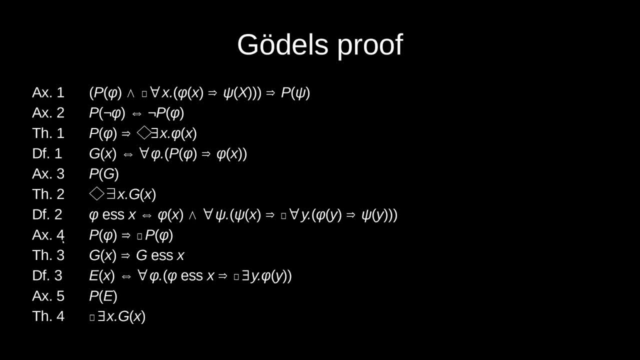 By definition, two of those essence. Axiom 5 defines necessary existence as positive, so that the one god that we found in theorem 2 now has this property of necessary existence, which means that all of its essences, including g. 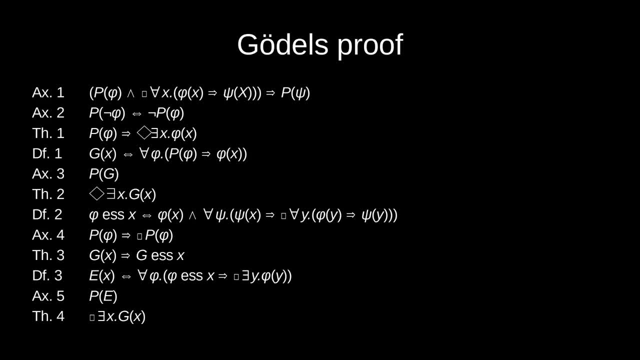 which means that this thing here now propagates the g over all universes, and then we get theorem 4, necessarily exists something that is a god. So to conclude, this video: does Gödel's god proof actually prove god? No, absolutely not. 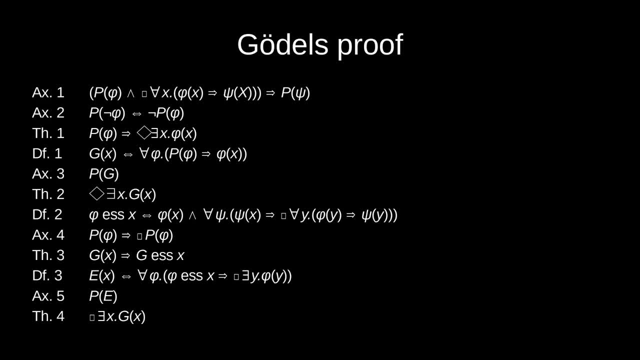 The axioms are extremely contrived and obviously specifically designed to produce the result: god exists. Many axioms are only there because without them the proof falls apart, even if they don't make sense. The formalities are quite trivial- much too trivial for Kurt Gödel. 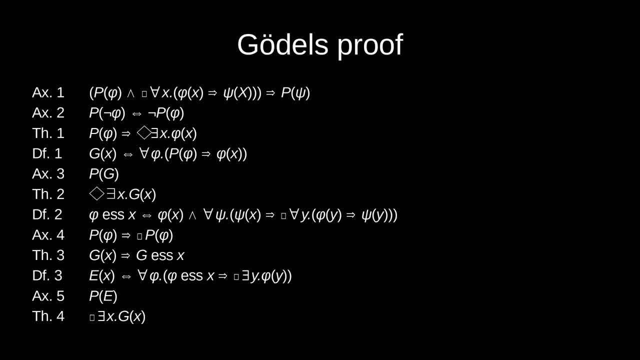 one of the greatest mathematicians of all time, to have worked 30 years on this, And even if all the axioms are true, in reality, this wouldn't prove god, Yahweh specifically, It would prove some god, and not even a single one. 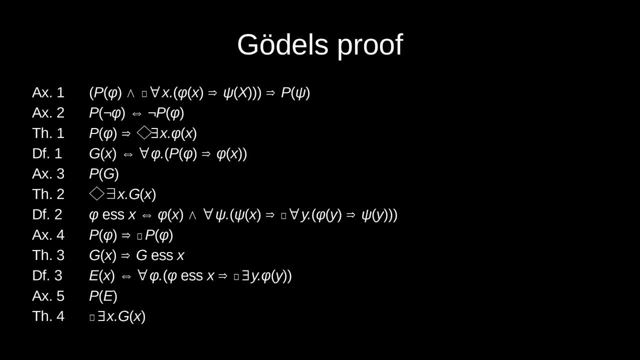 There could be multiple gods. It is only argued that Leibniz's law says: if two things have exactly the same properties- all the positive properties here- then they are the same thing. Well, I have two identical pencils. they don't turn into a single pencil just by being identical. 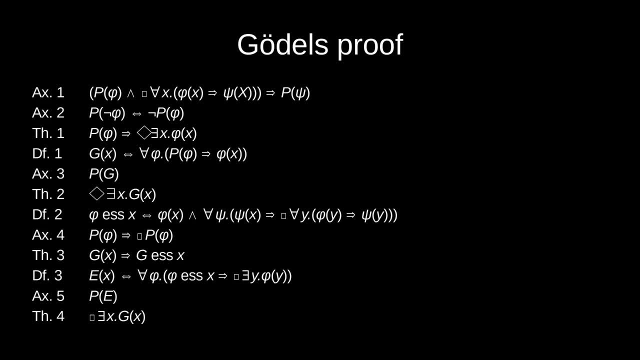 But I admit that this is debatable. But all in all, the proof is garbage And Gödel would have known that. so either Gödel meant this as a joke, like something he'd prank his colleagues with, or this is a hoax.